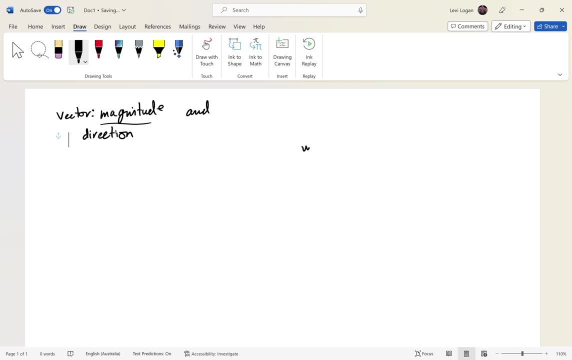 you can see applications is weight. so example: inclined planes. if you're standing on a surface, you have a force acting down due to gravity and you have the normal force acting up. so that's an example where you see vectors. you also have displacement and another big one is velocity. so you might be 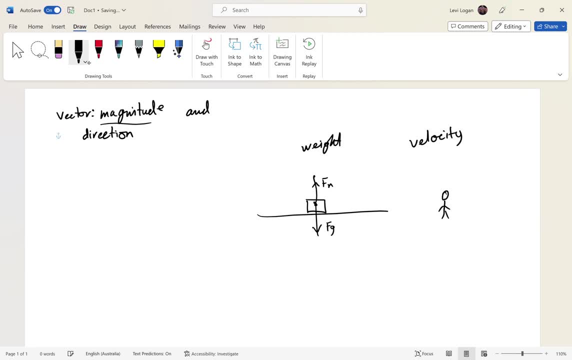 moving. a person might be moving a specific velocity in this direction, so they might have a velocity vector. okay, so those are some applications. I'm coincide with vectors. I think you need to know what a scalar is, so this is another important term. you'll see, in maths, a scalar- A scalar is a real 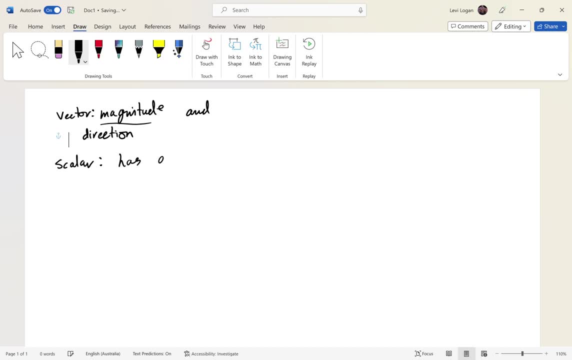 number that has a magnitude but no direction. So what do I mean by that? Well, the best way I like to visualize this is basically: what's the difference between speed and velocity? Now, this is a perfect example. so basically, velocity is a vector but speed is a scalar. So imagine you have a person here. 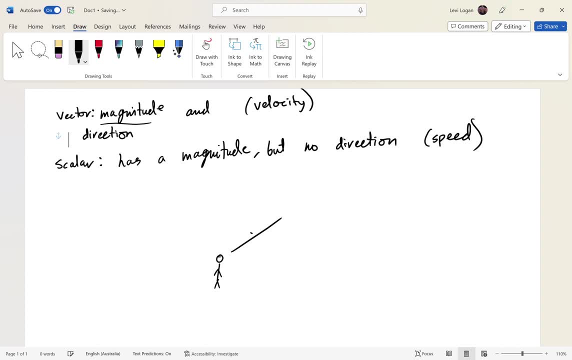 and he wants to travel with a velocity of three meters per second. For that to be velocity, he needs to have a direction. he's going in. Ok, If he just wanted to travel at three meters per second, if he just wanted to travel at that speed, he wouldn't have a direction. 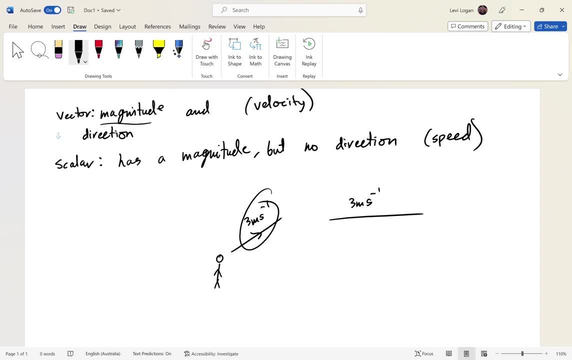 So basically a scalar is basically it's just a number, It's just multiplying. It's like saying, oh, you want to travel this fast, but you don't really care about the direction you want to go. Or you want to act this much force, but you don't really care about the direction. 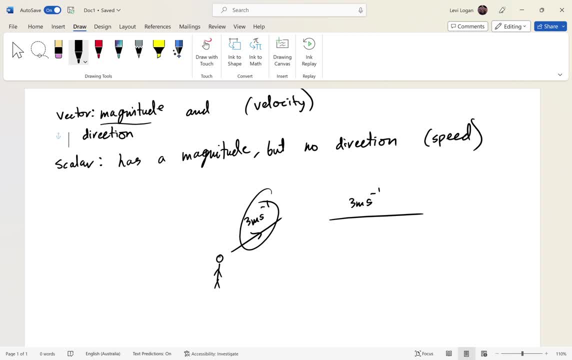 So basically a scalar is: it's a vector that doesn't have direction, It's just a magnitude, It's just a number, pretty much Okay. So that's what a scalar is. It's just a number. It's like multiplying something by a number. 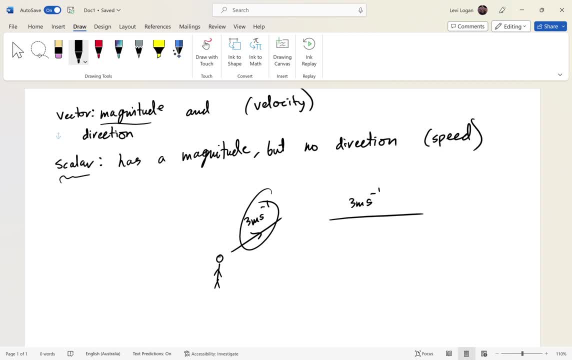 That's what a scalar is. That's why you see, like scale something by a factor of two. It just multiplies by a number. So a scalar is a number And a vector has magnitude and direction. A scalar just has magnitude, meaning it just has a length, a size, pretty much. 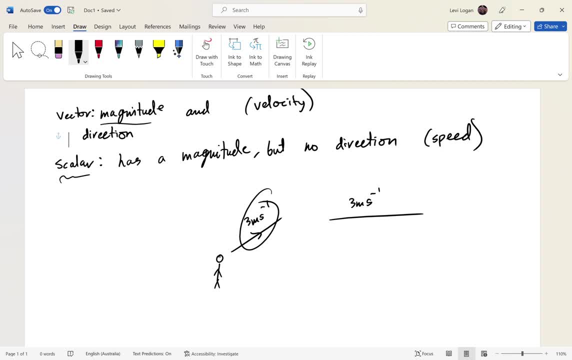 And that's corresponding to the number you pick. So a scalar, if it has a magnitude of two, that's a lot smaller than a magnitude of like a four, six or 10,000, pretty much All right. 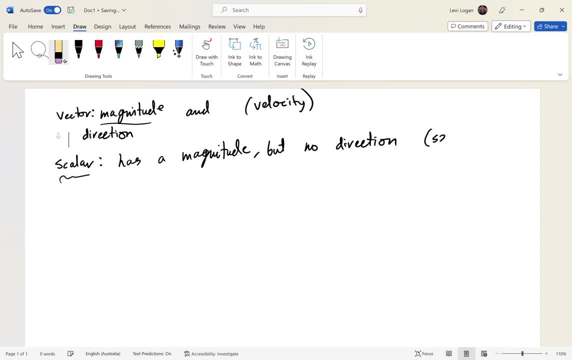 So that's just some basic stuff on what a scalar is. Let's go back and take a look at where and what a vector is again. So the best way I see a vector is it's just an arrow pretty much, It's just a line segment pretty much. 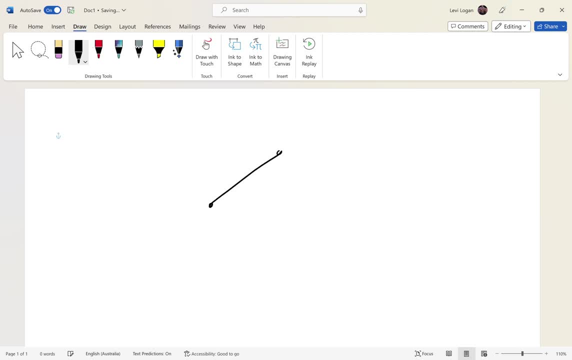 So it just goes from one point to another. Okay, And we denote it using these things here. This is the notation for vectors. So if you see this little arrow on the top here, that means vector, And they have this little subscript on the bottom as well to correspond for a vector as well. 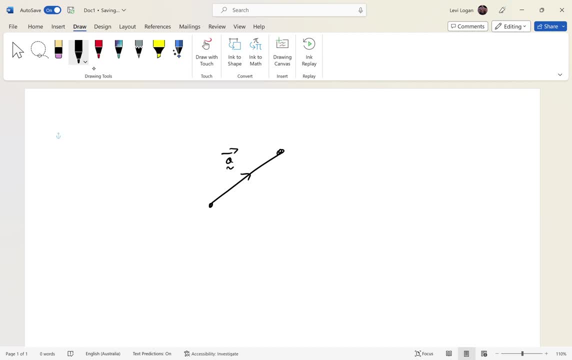 You also might see it written. It's written as like O to A. That we'll get to that in a second, But I just want to take a look at basically an example of a vector. So let's say we had the vector A. 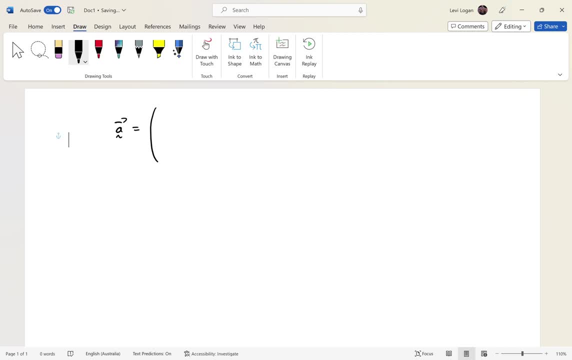 And the vector A has a horizontal component of one and a vertical component of one. So we can write them like this And basically like a column: So this top column means the X And this bottom column means the Y. So what does this actually mean? 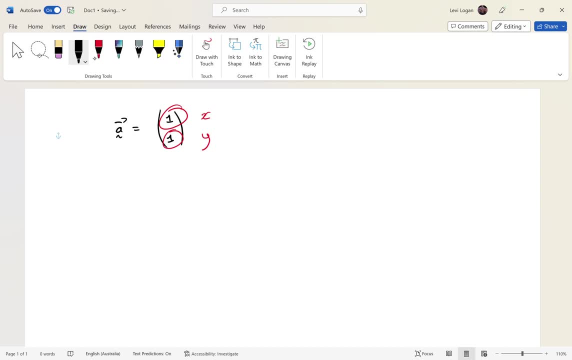 So what this vector is saying is that we have a vector that has a length of one in the X direction And it has a height of one in the Y direction, And these are both positives. So it's got this way and that way. 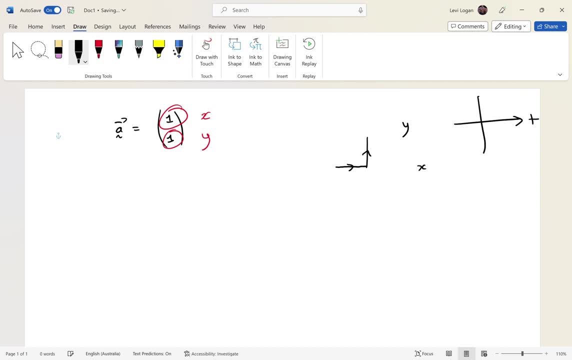 So just think of a coordinate system. You've got the positive this way And the negative this way. So this is for X and this is for Y. We use that when we're drawing our vectors as our orientation. So this here is the vector A. 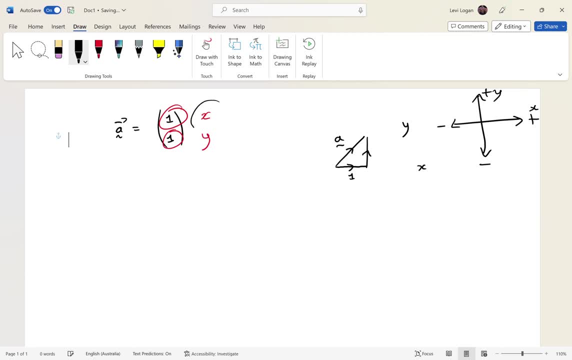 Because it has a horizontal component of one which is seen over here And it has a vertical component of one which is seen over here. Okay, So we write it as, basically, either as a column like this, Or you could write it like: 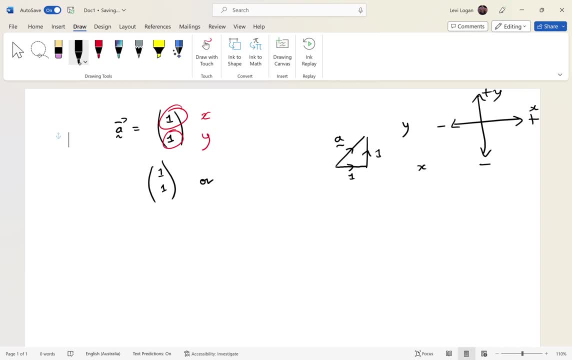 This is a new type of notation. You can have I plus J. Now what does that mean? Basically? that means there's just a one here. You can just write it A vector as like that, Or you can write it like this, If you want to be more simplistic. 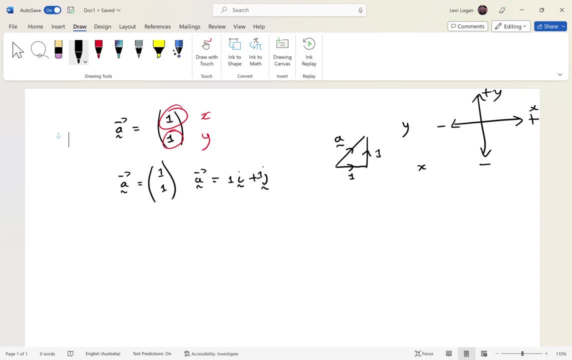 Right, Let's just get another. look at what this means pretty much, So I'm going to make another. Let's have a vector Q And it's going to have a. It's going to have 3 in the horizontal direction And negative 4 in the Y direction. 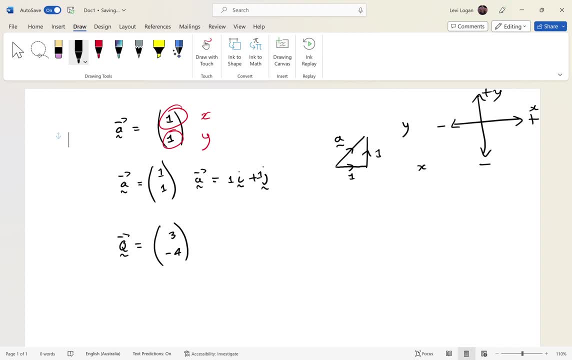 So what does that mean? So just looking, Focusing on our coordinate, Basically what our coordinate, our Cartesian system, looks like, Positive 3.. That's still. That's horizontal. So it's still going to be. So it's still going to be. 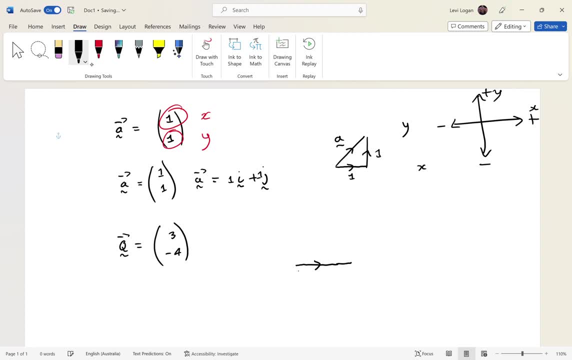 It's still going to be in the positive direction. So we're going to have a length of 3 here. Negative 4 means we have to go downwards, Because up is positive And down is negative, Just in two dimensions. So we're going to have a length of 4 downward. 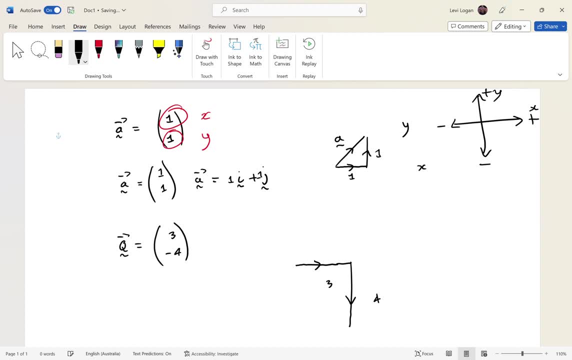 That's what we mean by that. Okay, So the vector Q has a direction of this pretty much, So it goes across 3 and down by 4.. And we could write a vector Q like this: So we're going to have 3i minus 4j. 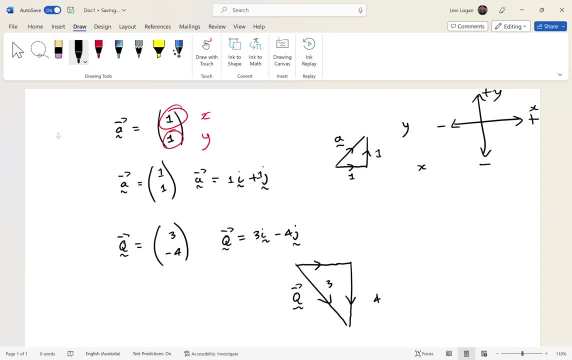 Okay, So we just We focus, We base our Base, our signs off, our Basically, our coordinate system, But we don't really have specific points a vector has to go through. So let's just consider our vector Q here And let's draw. 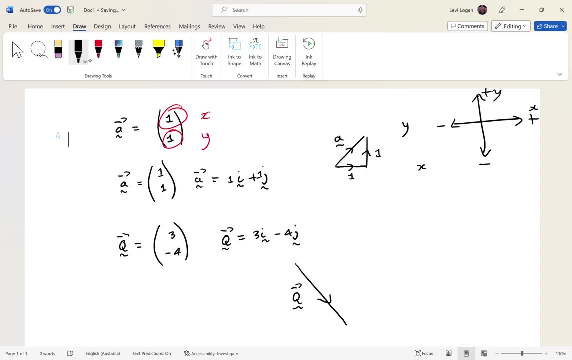 Let's just rub all that out. Let's just draw a bigger xy plane- So this is xy, That's positive and that's positive, So that's negative and that's negative. And let's just move a bunch of this stuff So we have enough room. 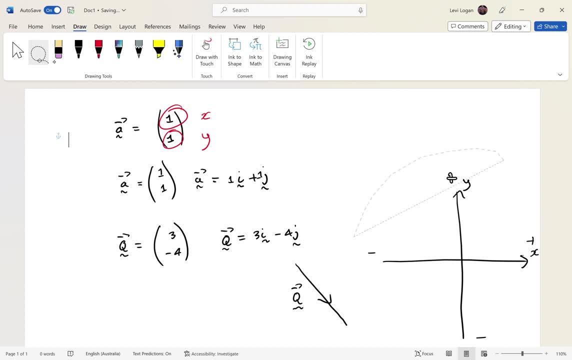 Basically it doesn't really matter, unless you make a vector. through certain points You can have a vector. Vectors can go anywhere, So this vector Can be here, Or it can be here Or it can be there. Oh, whoops. 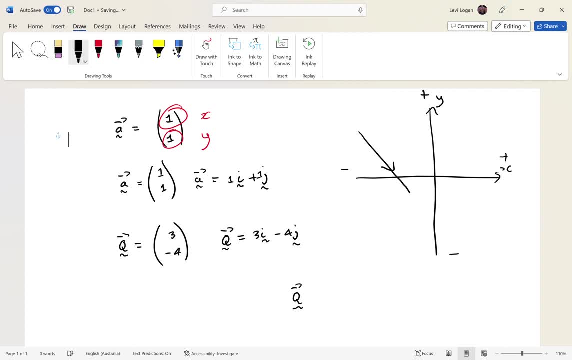 As long As its magnitude And direction Remain the same. Okay, So you can have a vector pretty much anywhere. It doesn't really matter where you place it, as long as it's constantly going. three units in the positive direction of the x-axis and four units in the negative direction of the y-axis. 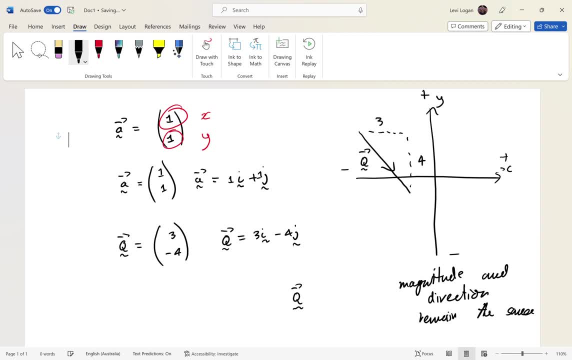 Okay, All right, Okay, So let's just rub all this out And let's get to. Let's get to adding vectors, pretty much because that's a more useful thing. you'll need to do With vectors. You might be asked to draw them. 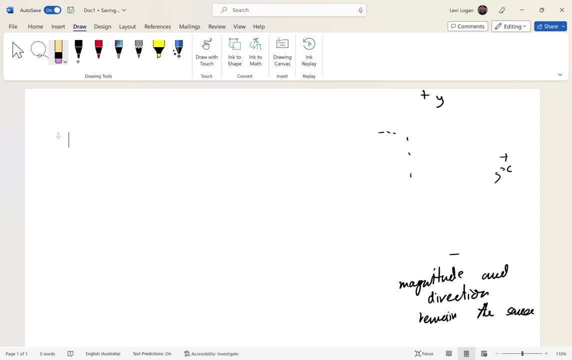 But that's quite easy. So they're more likely to ask you to add vectors. Okay, So I'm going to add the vectors, basically algebraically and geometrically, So I'm going to get. I've prepared some two vectors before. 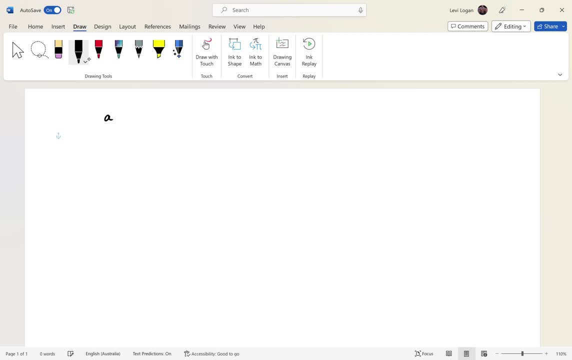 So consider the vector A And it has. It's just that It just goes 1, 1.. And consider the vector B, And it has. It goes negative 1 in the x-direction and positive 4 in the y-direction. 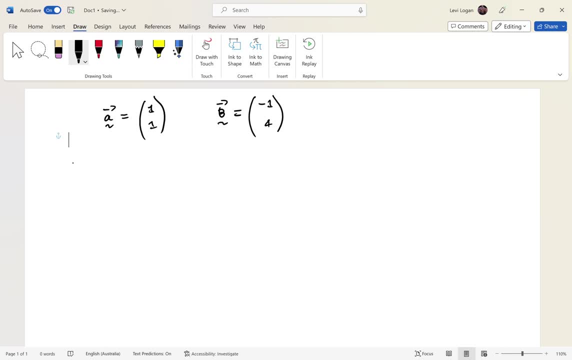 All right, I want you to find what the vector A plus the vector B is, Okay. I want you to give it in column form And I want you to draw a picture, Okay. So feel free to pause the video And have a go. 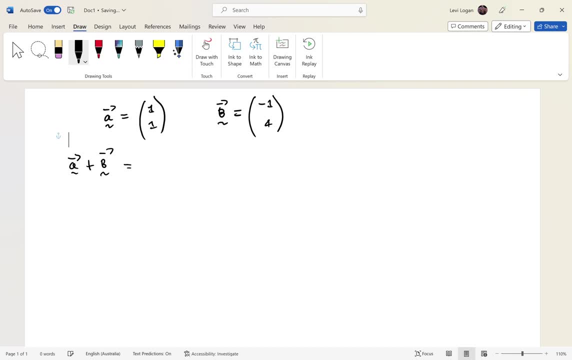 All right. So what I'm going to do, I'm just going to write our vectors here. So we have vector 1, 1.. Which is our A vector, Plus our B vector, Which is negative, 1, 4.. 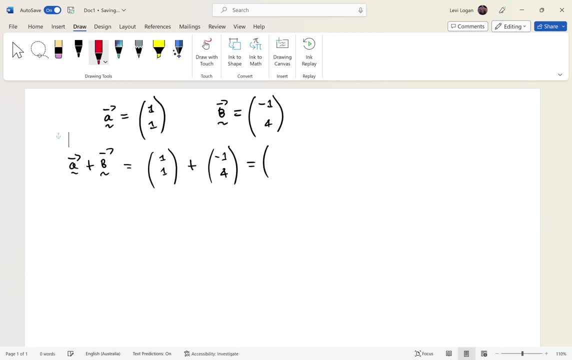 Okay, So that's going to be. You just add the x's with the y's, So the top one is going to be 0.. And the bottom one is going to be 5.. Okay, So our vector A plus B. 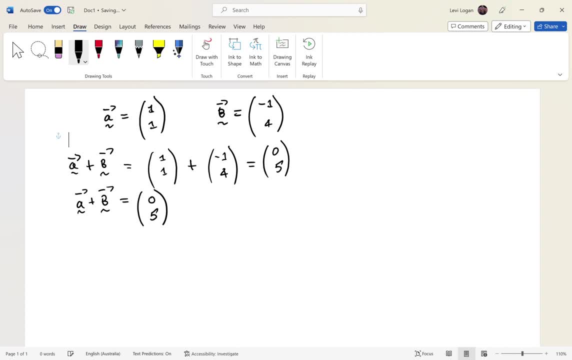 Is equal to 0, 5.. So now let's just draw a picture. So I'm going to draw the vector A. The vector A goes one unit across And one unit up. Okay, So that's our vector A. I'm going to get rid of these bits. 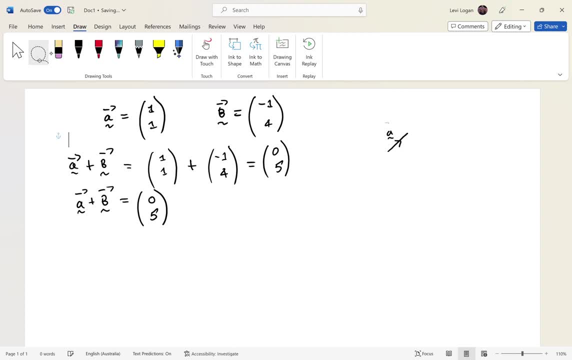 So this is A. Put that on that side. That's the arrow there, All right? Actually, no, I'm going to make this a bit bigger. So that's our vector A And our vector B. So our vector B goes negative 1.. 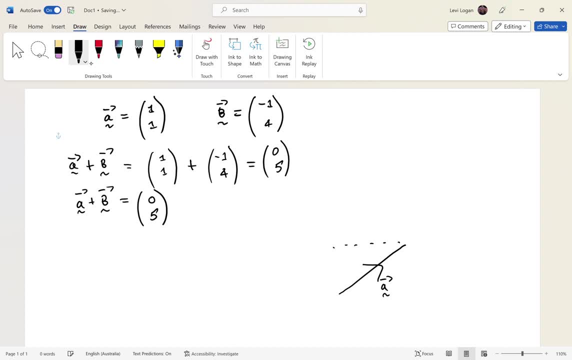 In the x direction And it goes 4 up. So it's going to be looking like this: Okay, So this is our vector B, And what I've done Is basically, when you add vectors, You add head to tail Pretty much. 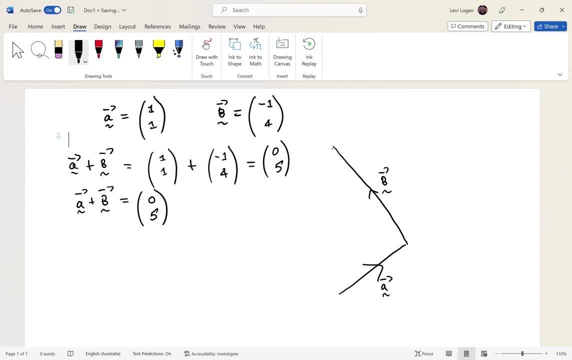 Okay, Geometrically, So you can see, This is the head of my vector A And this is also where the tail is of my vector B, And basically, what we're trying to find Geometrically Is this here: This is vector A. 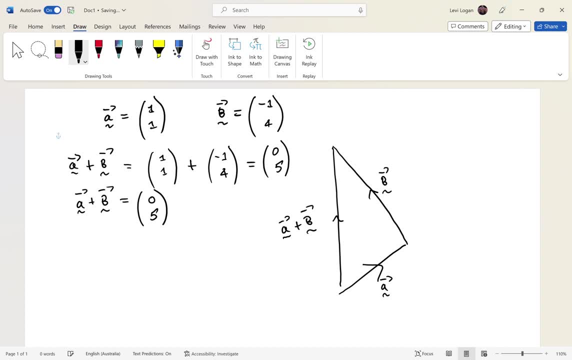 Plus B. Okay, So vector B Is negative: 1, 4.. And vector A is 1, 1.. And we just added that before And that gives us the vector 0, 5.. Now, geometrically that makes sense. 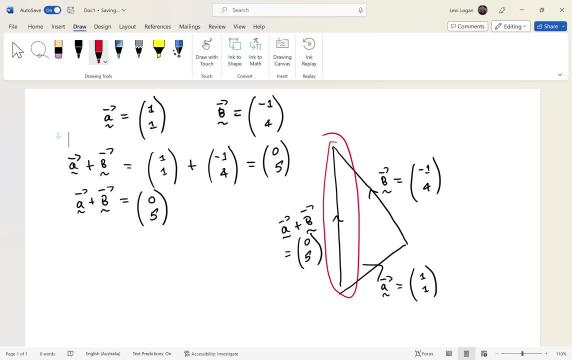 Because this vector Doesn't really have any horizontal component. It doesn't at all. It's got 0. And it's straight up. This vector appears geometrically longer than B, So It satisfies Pretty much What we were thinking earlier. 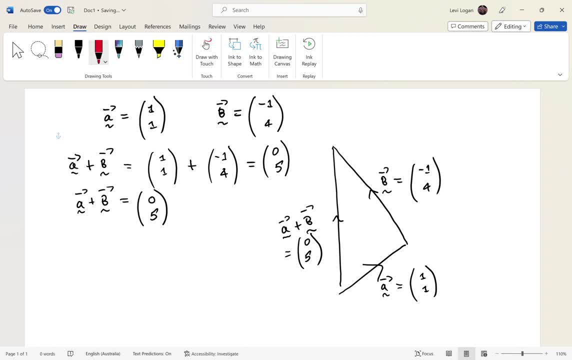 Over here With these ideas here. So that makes That's what it is: to geometrically add a vector. Okay, Alright, So I'm going to rub all this out And I'm going to give you Another example. Pretty much. 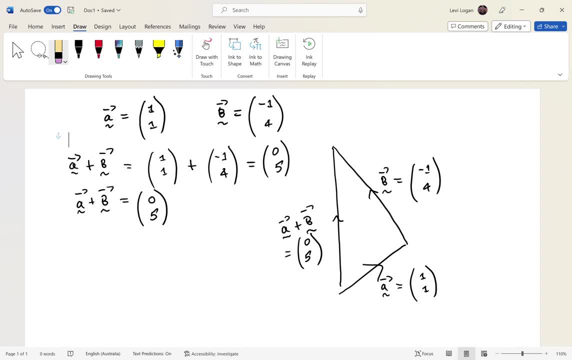 I want you to do the exact same thing we just did with that problem. I want you to First off Find The vector Here, And I'm going to give you Another example. Pretty much I want you to do the exact same thing we just did with that problem. 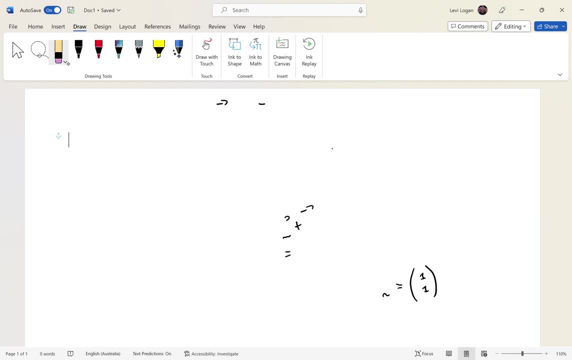 I want you to, First off, Find The vector We're trying to find And I want you to try and draw a picture of what's actually You're Looking at. Okay, So let's say we have the vector. 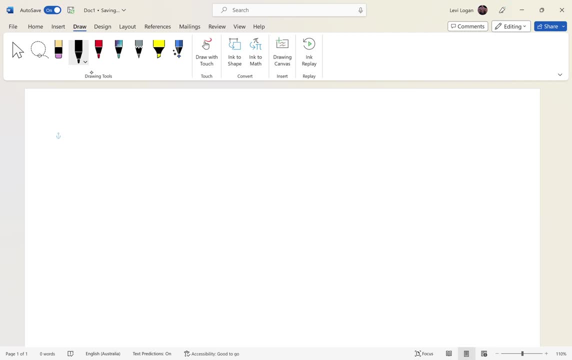 A Again, Except it has It goes Negative 2 in the x direction And 5 in the y direction And we have the vector B And it goes. Let's go 6 in the x direction. 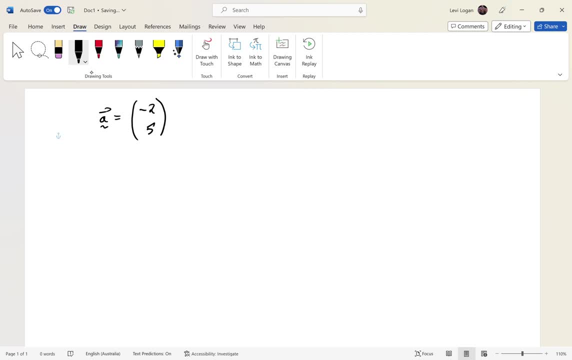 And 5. In the y direction, And we have the vector B And it goes. Let's go 6 in the x direction And 5. In the y direction And 6. 4.. 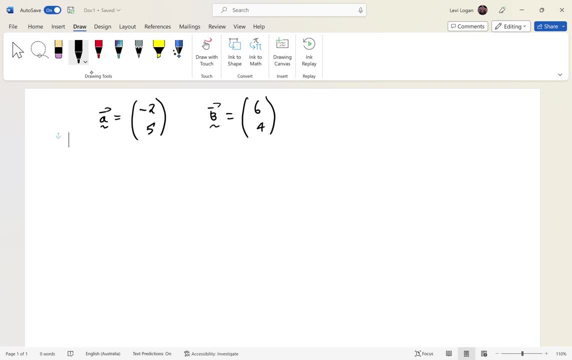 In the y direction. So I want you to Find The vector A Plus B And I want you to draw a picture. Okay, So feel free to pause the video, All right? So first thing we're going to do: 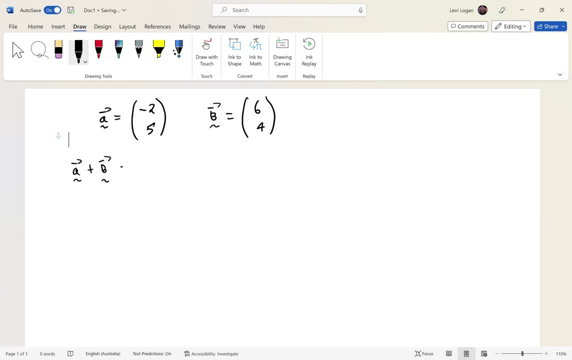 Is going to write our vector A So negative: 2., 5. Plus 6. 4.. All right, All we got to do Is add: our x Is Together And 5. Plus 6.. 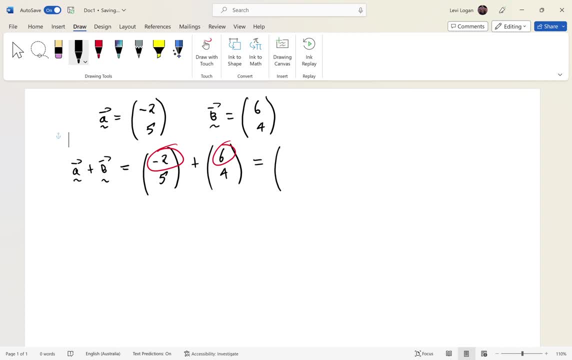 So our top of our column Is going to be Negative: 2. Plus 6.- That's 4.. And we're going to add our bottoms And 5. Plus 4.- That's 9.. Okay, 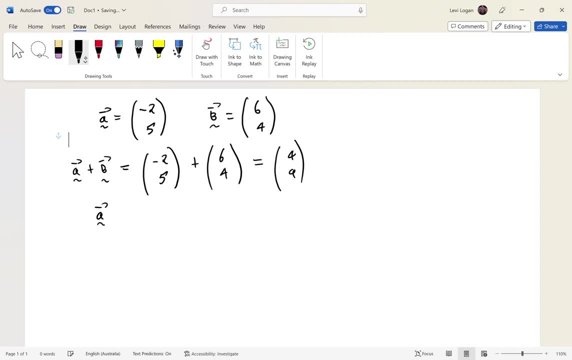 So that is. That is the vector A Plus B. It is Goes: 4. Across In the x direction- Positive Direction- And 9. Vertically In the positive direction. All right, So I'm going to draw the vector. 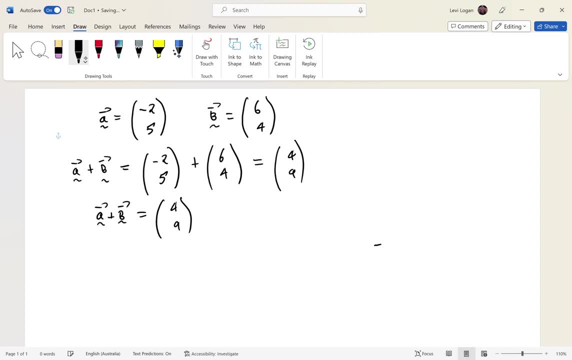 A. So the vector A Goes 2. In the negative direction And goes 5. Positive. So it goes 1., 2., 3., 4., 5.. So that is our vector. 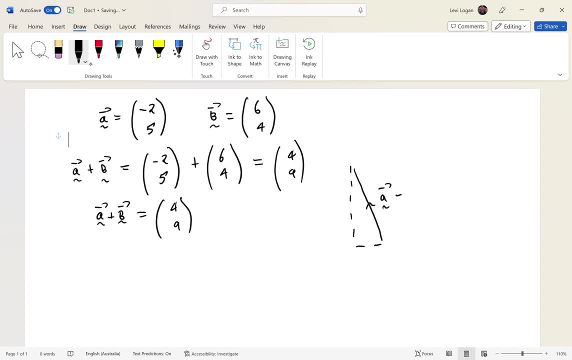 Oh, That's a terrible arrow. That is our vector A. Okay, So equal to Negative: 2., 5. And I'm just going to get rid of these Now that I've drawn it- Um, A. 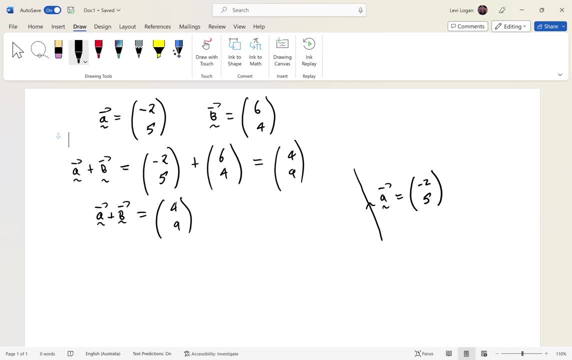 B Vector. I'm going to draw them, Not joined together Straight up, I'm going to move them together. So I'm going to draw a vector B. Uh, Vector B, It goes 6.. In the 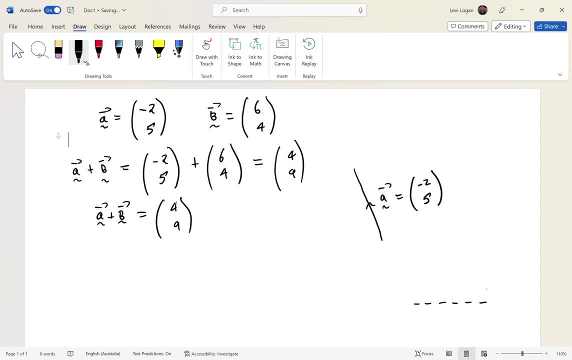 Um Positive X Direction, Goes 1., 2., 3., 4., 5., 6. And goes 4. Up. So That's our vector B. Oh, Whoops, Okay. 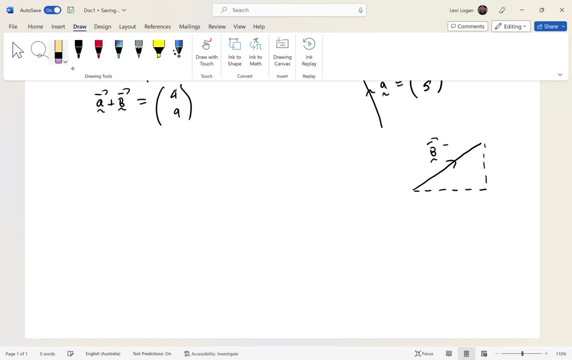 I rubbed that out now, So that's our vector. Oh Gosh, I rubbed it all out together, So let's just say That's our vector B. Okay, All right, So when we add vectors, We're going to go. 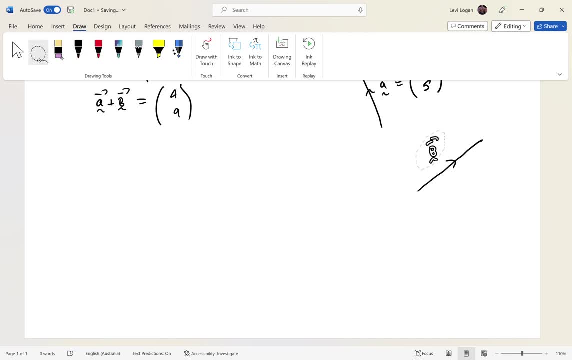 Add head to tail. So This is the Tail of the A Vector And this is the Head Of the A Vector. So All I'm going to do Is just I'm going to move. 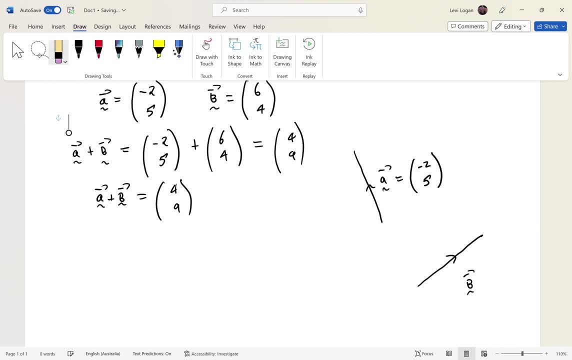 This Here, So It connects up. Boom, That's our vector B, And our vector B Is 6. 4.. Okay, So This Here Is Our Vector B. Okay, 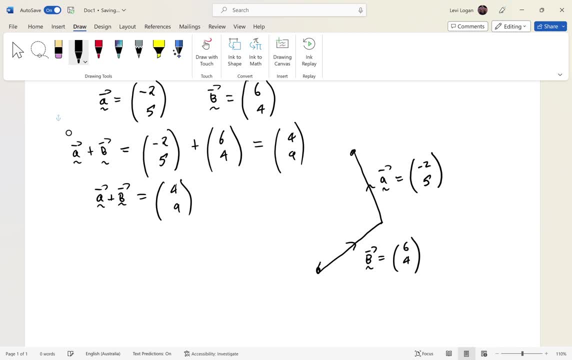 So This Here Is Our Vector A Plus B. Okay, And Yeah, That's Pretty much Our Geometric Feature. So This Vector Here Is 4. 9.. 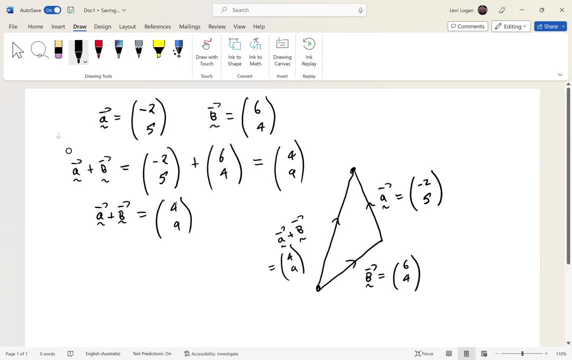 And That's Pretty much It As Well. All right, So That's How To Add Vectors. Okay, Now Let's, Let's Rub All This Off And 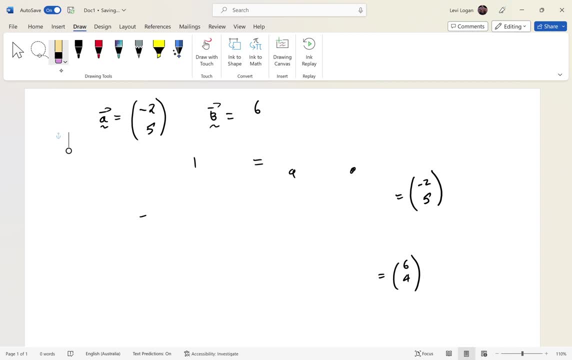 Let's Take A Look At What Happens If We Subtract Vectors. Okay, So There's No Such Thing. That Is A Minus Vector B. 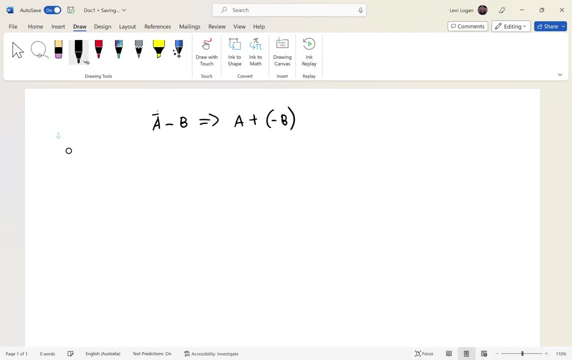 What We Like To Think Of It Is Just A Plus The Negative Vector Of B. So These Are Vectors. That's Pretty Much So What? 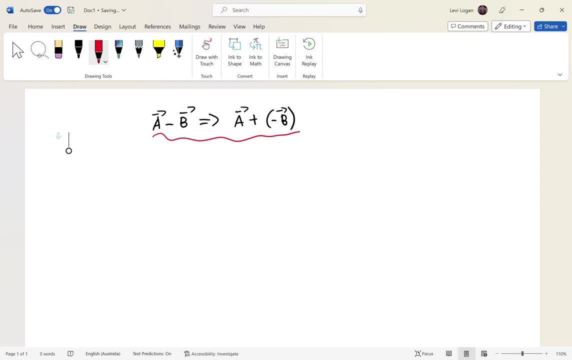 Do I Mean By That? Okay, All Right. So Let's Say, Let's Say You Had The Vector. Um, Let's Just Draw A System, Let's. 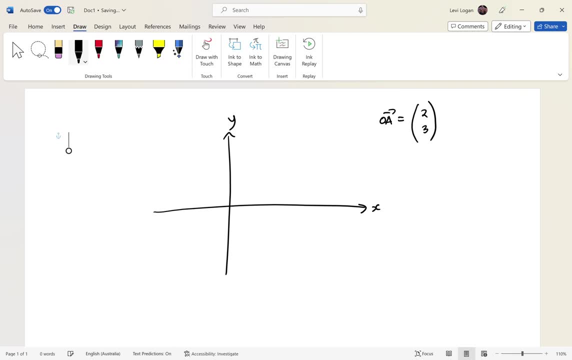 Draw A Corner System. So O To B Is Equal To Four Negative One. So O Is Our Origin And The Point A Is The Point. 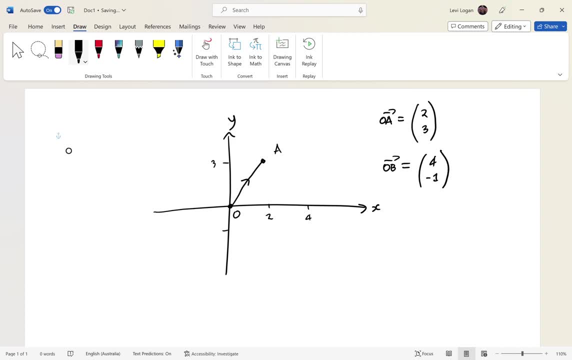 Two, Three. So That's A. So That's Our Moving, Our O On This Side. That's Our Vector B. Okay, All Right, Now Let's Say: 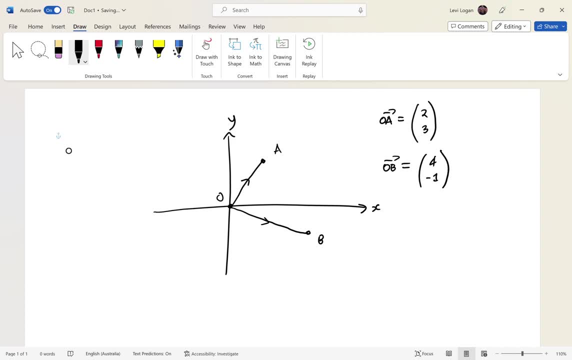 We Wanted To Find Um The Vector Here. So The Vector A To O Is Our Origin And The Point Is Our Origin. So We Wanted 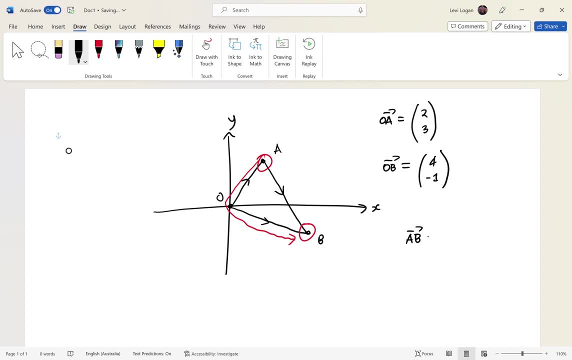 To Find Our Vector. So We Wanted To Find Our Origin, So We Wanted To Find Our Vector. Is A To O, So Recall The Vector. 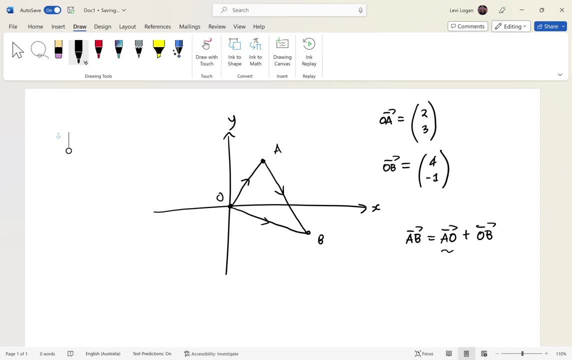 Depends On Direction And Magnitude. So This Is The Vector O To A. So If You Want To Find Our Vector, So Knowing This, We 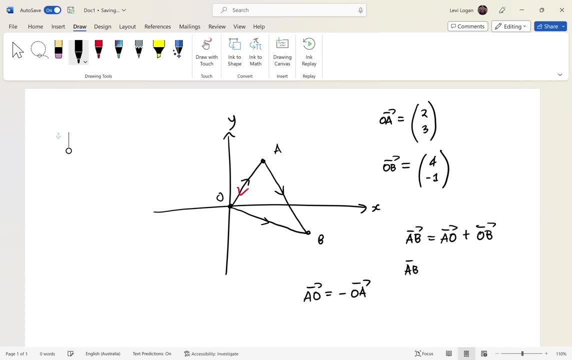 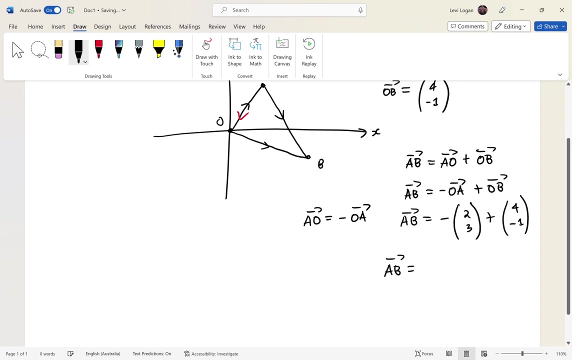 Can Replace That Fact In This Equation Over Here. So We Have A To B Is Equal To Negative, O To A Plus O Is Equal. 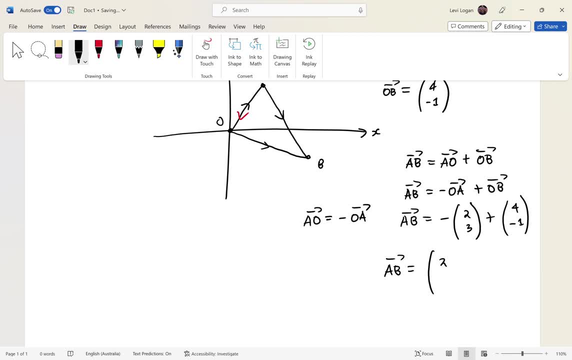 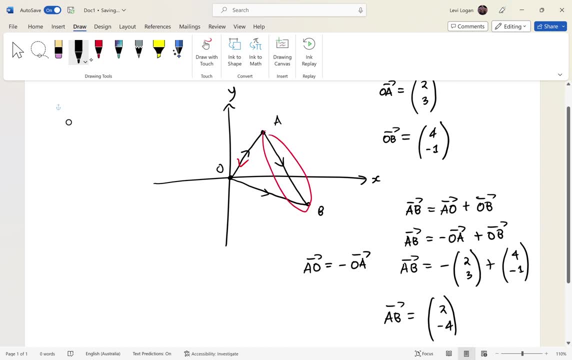 To Negative. Two Plus Four Is Just Two Negative Three Plus Negative One Is Negative Four. So This Vector Here Is Two Negative Four Right. So 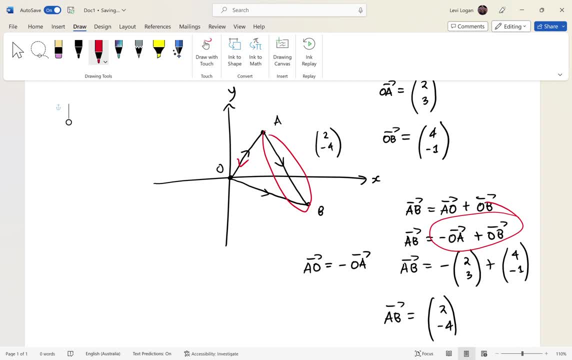 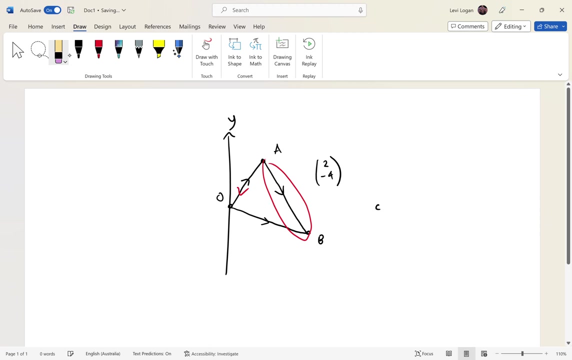 You See, All Right, Um, I Hope That Made A Bit Of Sense. I'm Now Going To Do Another One, So I'm Just Going To 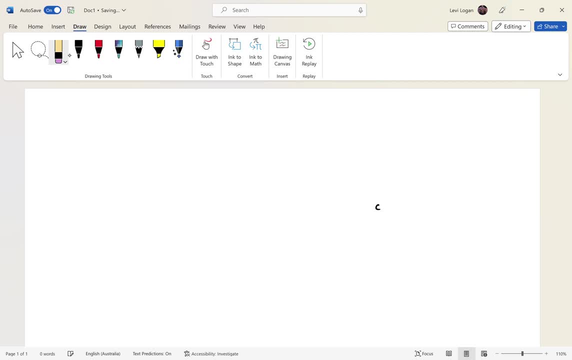 Rub This All Out. If You Had The Vector, Um Oh, Let Me. I'm Just Trying To Think Of One On The Spot Because I've 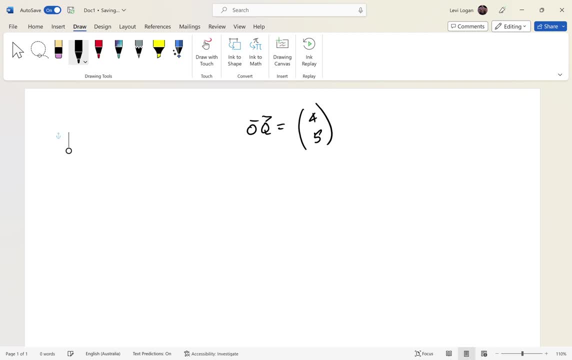 Done All The Stuff I Want To Do In This To Be, And You Had Six And Seven And Let's Say I Wanted To Find 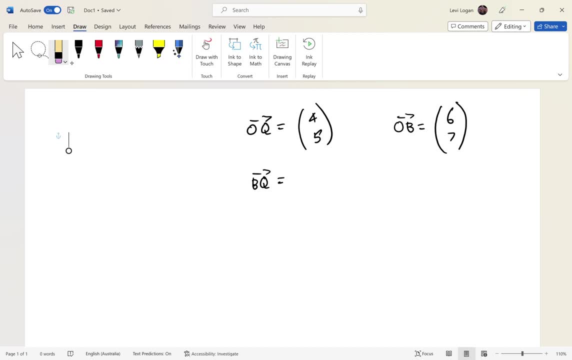 The Vector B To Q. Okay, So Feel Free To Pause The Video And Have. This Is Just An Arbitrary Diagram Of What's Going On. 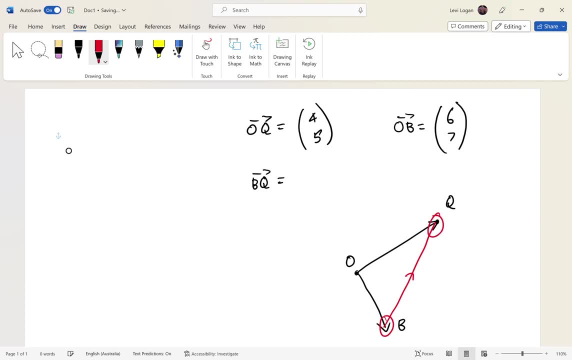 So This Is The, This Is O, This Is Q And This Is B. Okay, You Want To Find B To O Is The Same As. 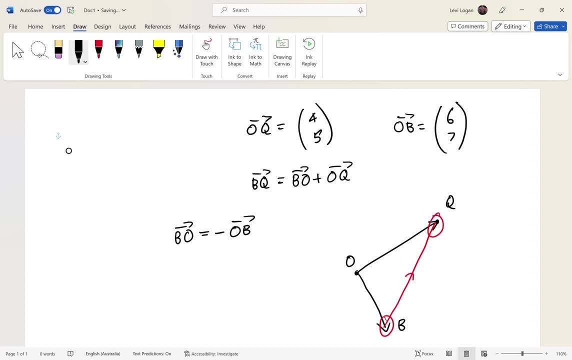 The Negative Vector As O To B, Because It's The Same Vector- Is Just Going In The Opposite Direction. That's Why We Say So. 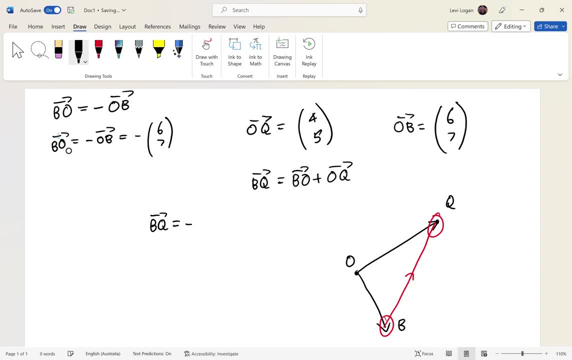 B To Q Is Equal To Negative, O To B- Okay, Plus O To Q. So That Is B, Q Is Equal To Negative, Six And. 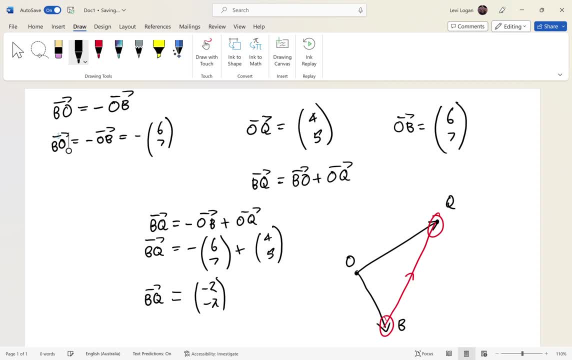 Seven Plus. So This Vector Here Is Negative Two Negative Two Right. So This Is Just An Arbitrary Diagram, Because When I Draw, When I've 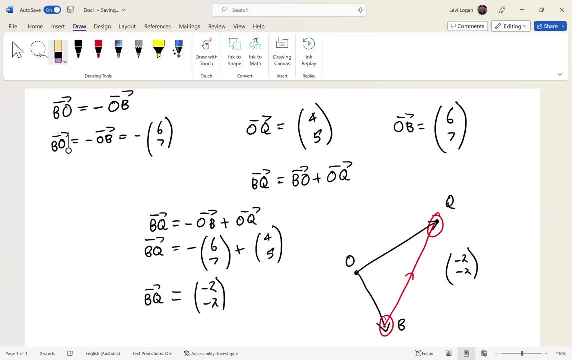 Drawn This. It Looks Like To Draw This Properly, You Would Need To Draw An X Y Plane, So I Just Draw A Little X. 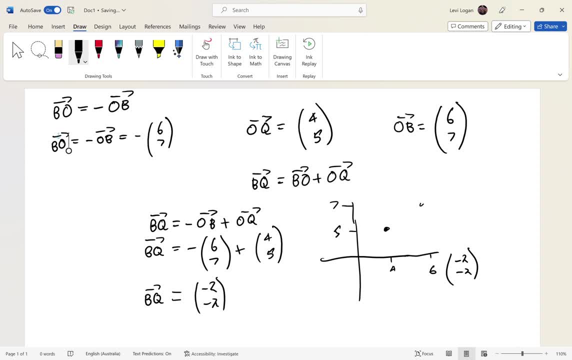 Y Plane, You Would Need To Plug In The Corresponding Vectors, And The Vector You Found Here Is Just This One Here, So That Vector.